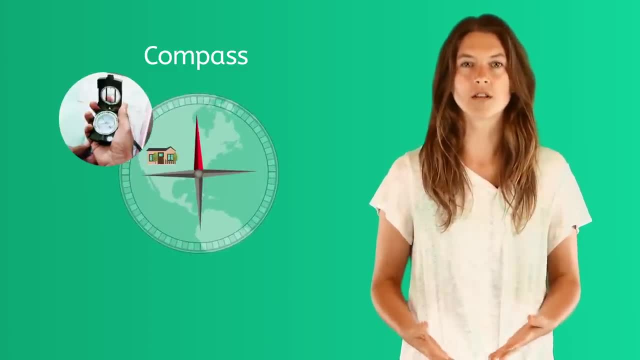 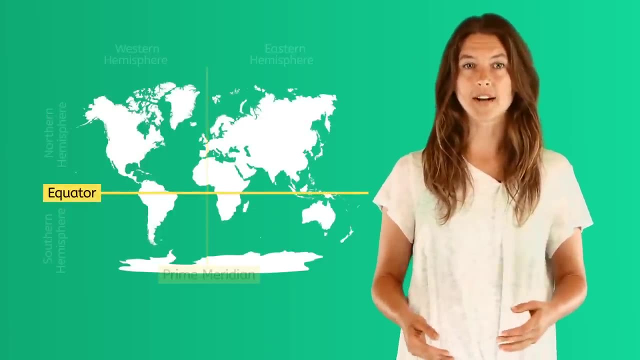 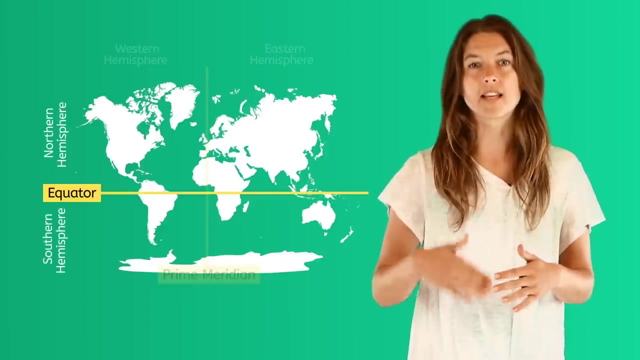 tells the direction of things like where your home is found in our world. our world is further divided into four main sections called hemispheres. the equator is an imaginary horizontal line around the center of the earth. it divides the earth into the northern and the southern hemispheres. 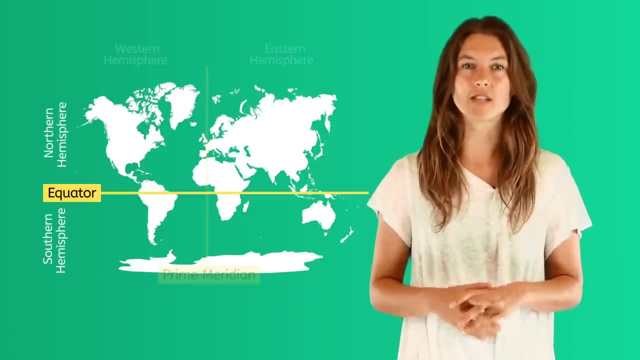 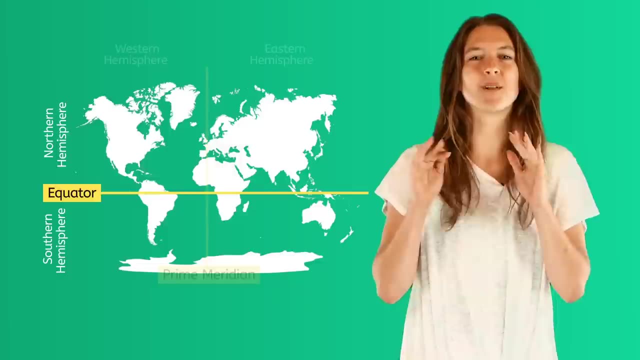 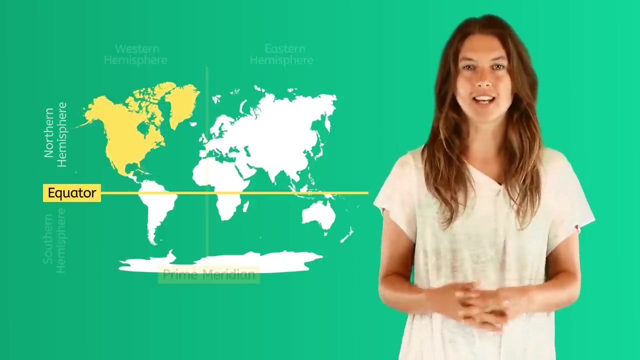 all continents, countries and oceans are divided into the northern and the southern hemispheres. the oceans found above the equator are considered to be in the northern hemisphere, and continents, countries and oceans located below the equator are considered to be in the southern hemisphere. North America is located in the northern hemisphere. 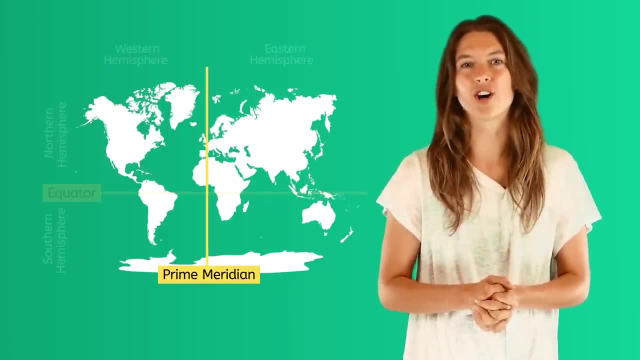 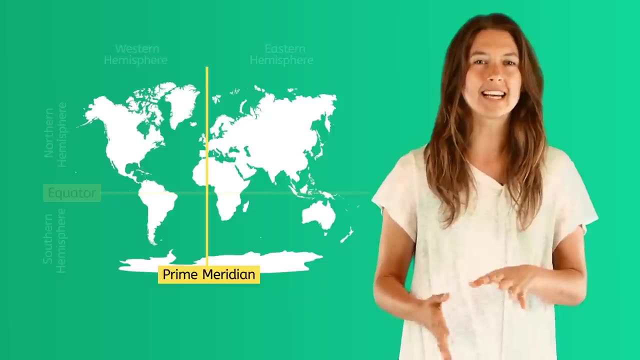 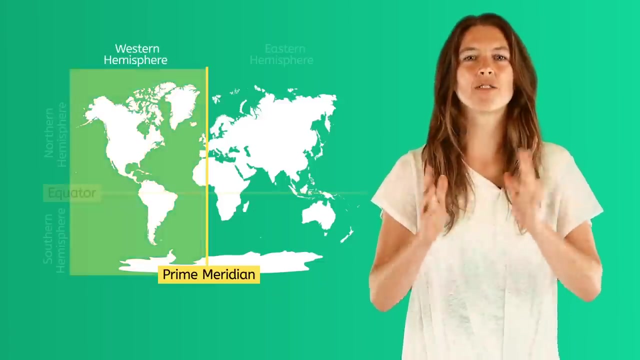 the vertical imaginary line through the center of the earth is called the prime Meridian and it divides the world into the eastern and western hemispheres. you can guess where the continents and countries to the west of the prime Meridian are located. yes, in the western hemisphere. so that means that. 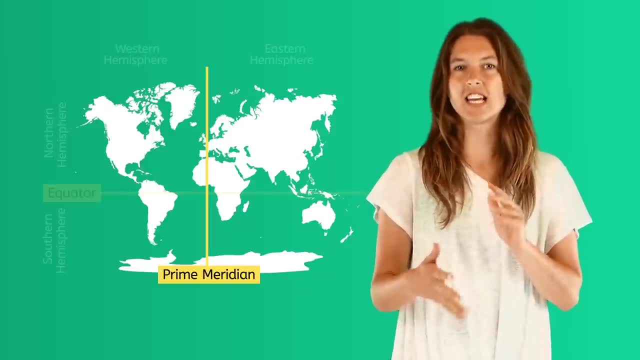 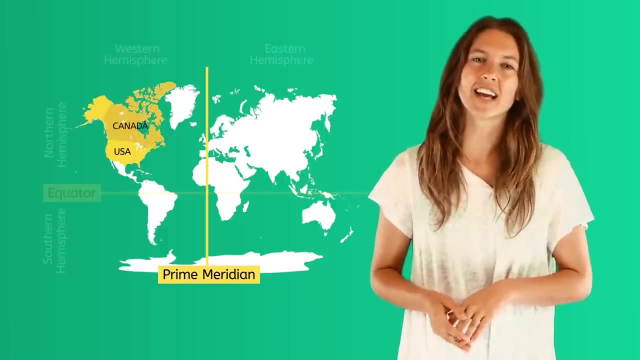 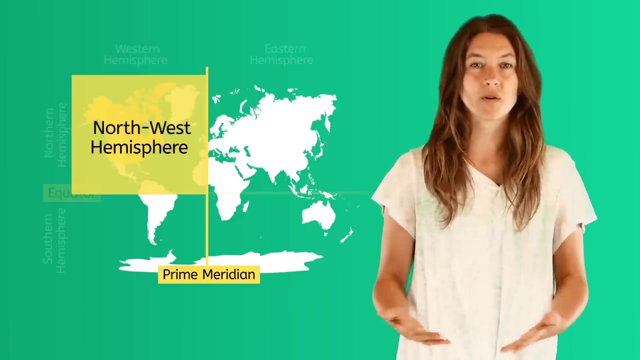 continents and countries located to the east of the prime Meridian are in the eastern hemisphere. super the USA and Canada are located in the western hemisphere. actually, we say they're in the Northwest hemisphere because they're in both hemispheres. cool huh, hemisphere lines might be. 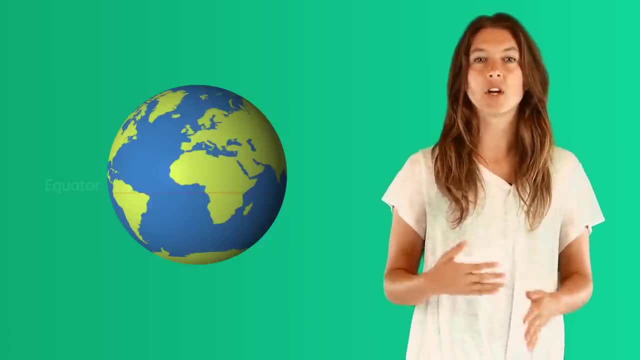 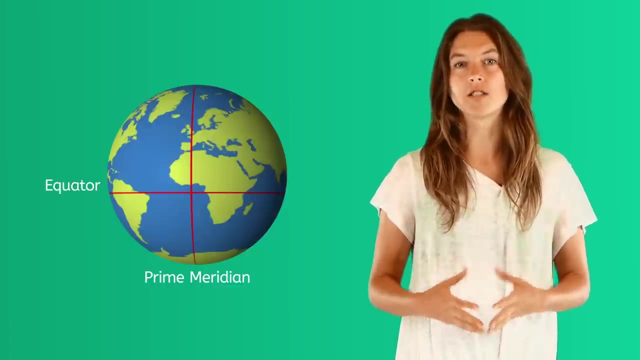 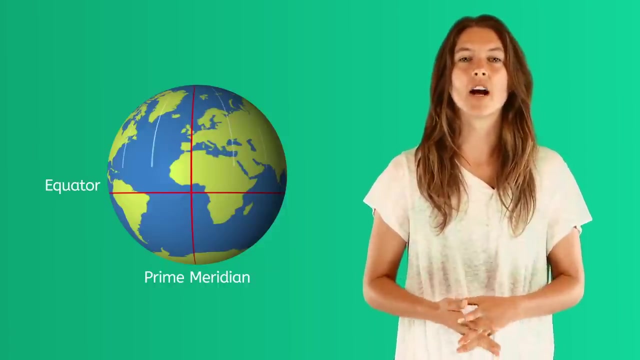 cool on Earth, but they are actually drawn on maps now. the equator and the prime Meridian aren't just randomly placed around the Earth. scientists who study the Earth are geographers. agreed many, many, many years ago on a system of more imaginary lines that run up and down or north to south along the 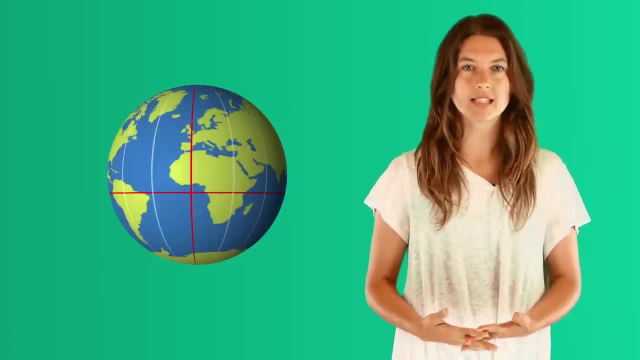 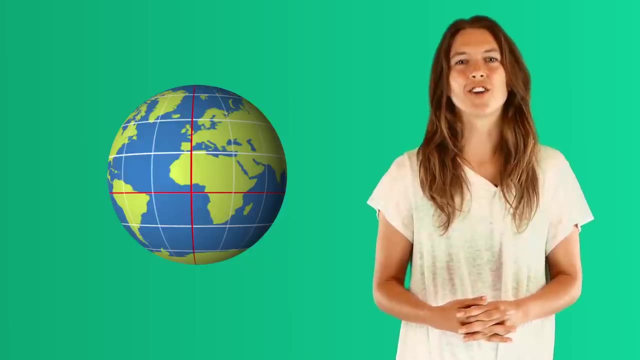 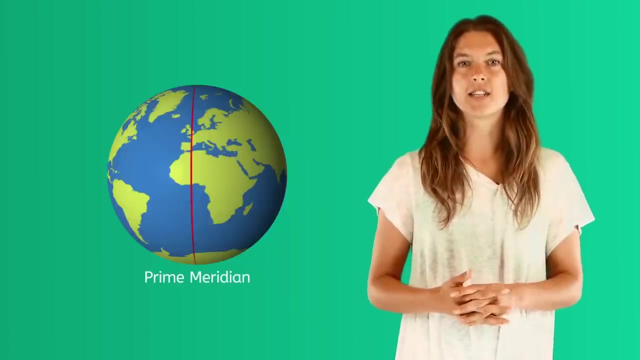 prime Meridian and they agreed upon a system of lines that ran east and west across the Earth in the same direction as the equator. these lines are called lines of latitude and longitude and they are measured in degrees. the prime Meridian is considered to be at zero degrees longitude around the opposite side of the 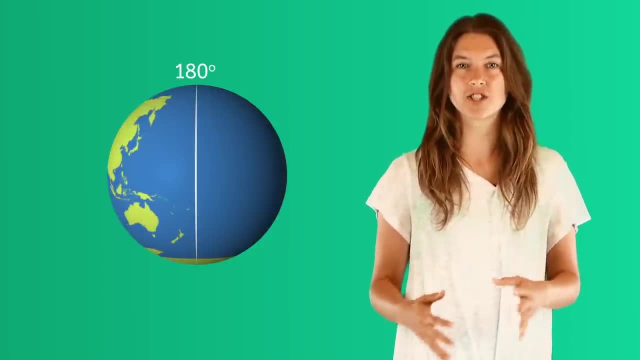 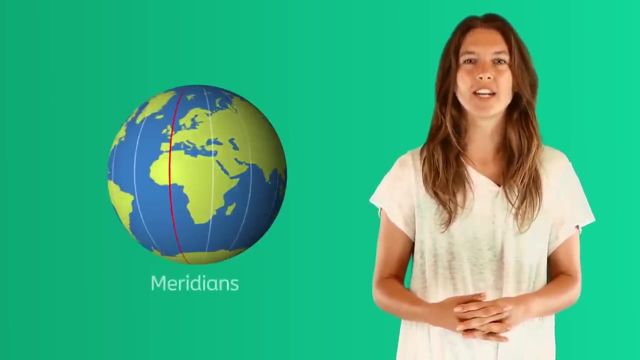 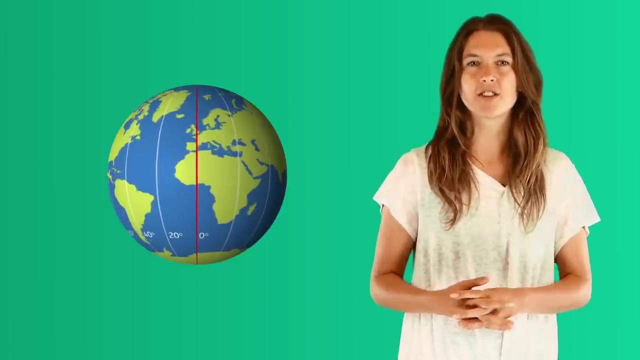 prime Meridian, the longitude is 180 degrees longitude. then all that space is filled in with more lines of longitude called meridians. each line equals one degree, with each of the degrees going around the world from zero to 360.. can you guess why that's right? it's because the distance around